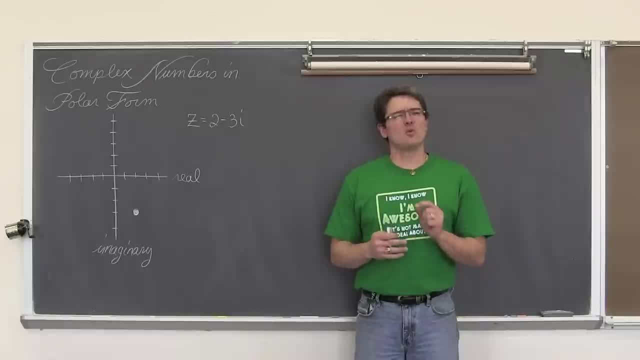 video introduce the DeMoivre's Theorem, which hopefully I am not butchering that name too much- and which will show us how to take complex numbers in polar form and raise them to a power and find a root. But for right now let's get the basics down. We have a number, a complex 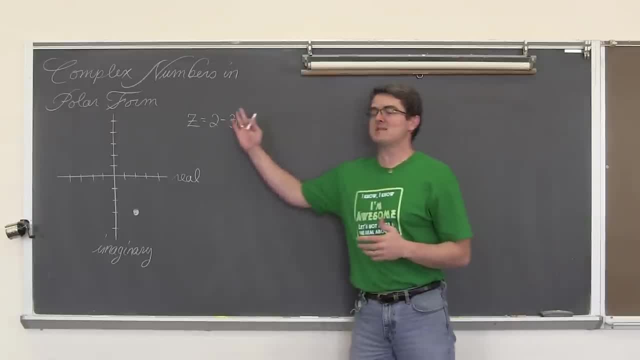 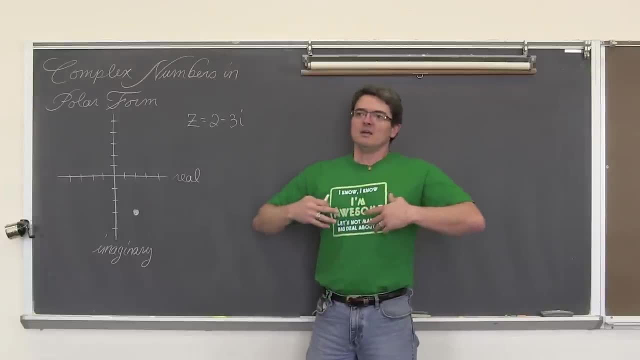 number, and it is 2 minus 3i. We would say that that was in rectangular form. I have that point displayed on a rectangular coordinate system. Well, actually it is rectangular, but it is the imaginary plane where the horizontal axis, instead of being what we would normally, 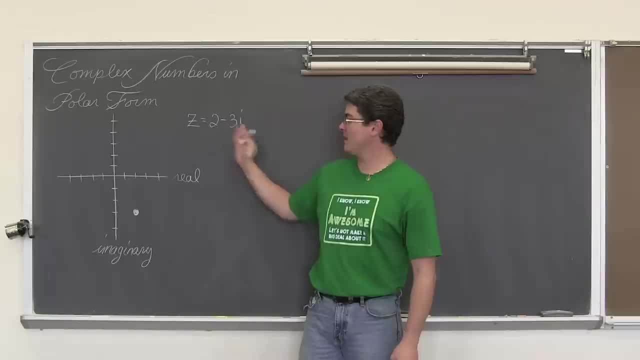 think of as the x axis is the real component of the complex number And the vertical scale is the imaginary part. So we have got 2 minus 3i displayed as going from the origin right 2 and down 3. Just like we would do if this were just a simple rectangular coordinate. 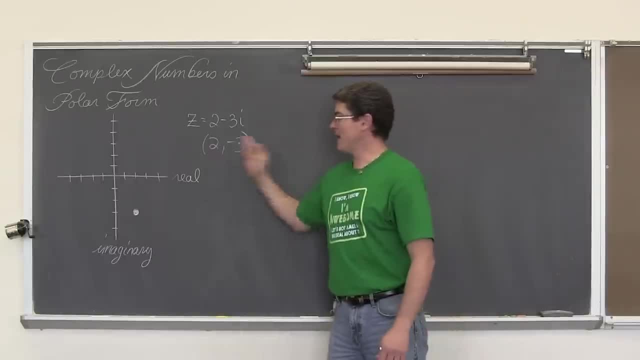 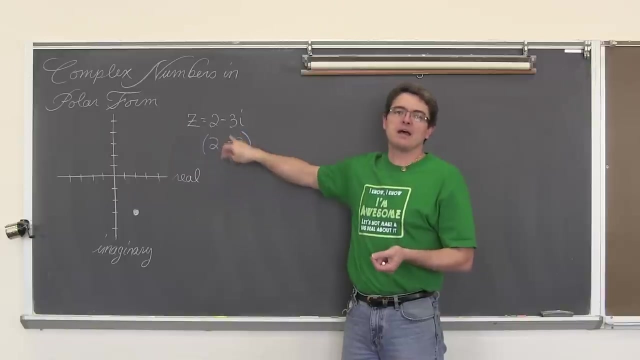 of 2 minus 3i, Where you would go Right 2 and down 3.. So when you are looking at complex numbers, the real portion of the complex number acts kind of like your x coordinate would and the imaginary coefficient is going. 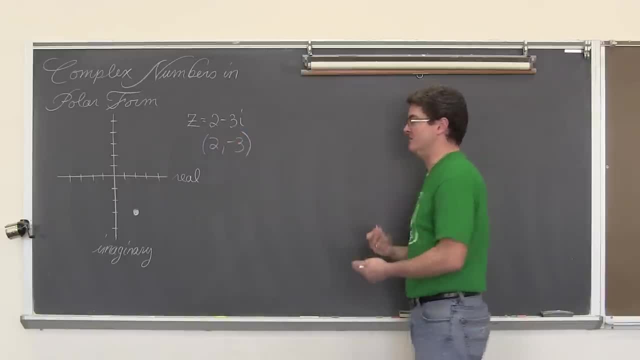 to act as your y coordinate, Just as a tie in. So the real value is horizontal and the imaginary coefficient is your vertical component, Which we have known up until now as y, but it is b. Ok, So we want to find the absolute value of z And a formula for finding the absolute. 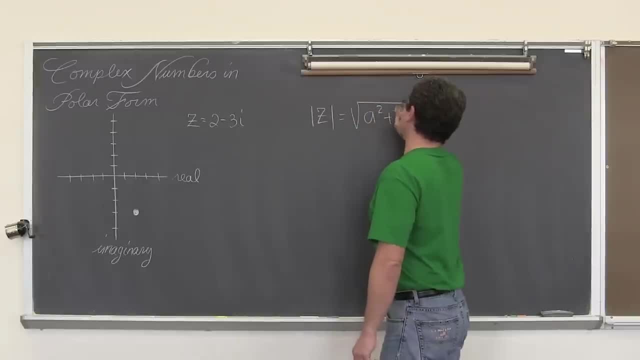 value is the square root of a squared plus b squared. Well, you might be going- that looks very, very familiar- to another formula I have learned, Which is: r is equal to the square root of x squared plus y squared. You would have seen this formula in a previous video. 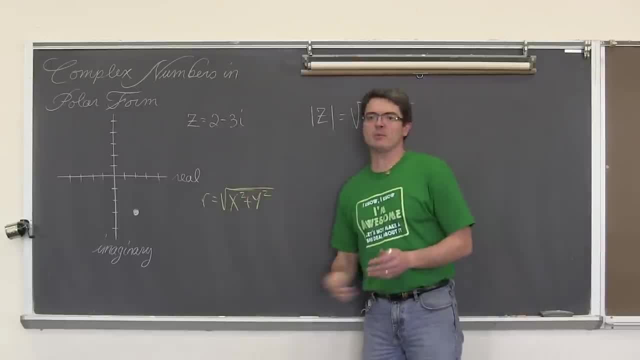 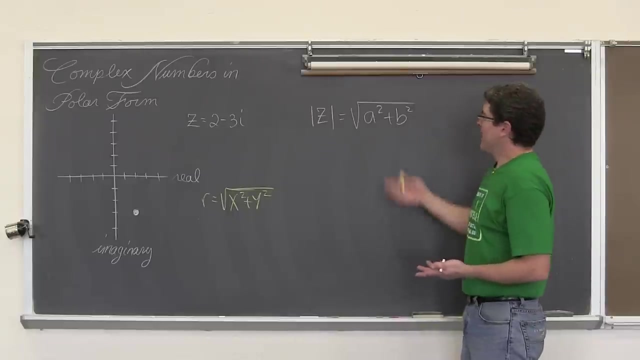 Well, you have seen it probably since you started studying trigonometry, but we just did a video about converting between polar coordinates and rectangular coordinates And you know converting points and equations. This formula was in those videos, That is, and it is basically the Pythagorean Theorem, really, And these two formulas look exactly. 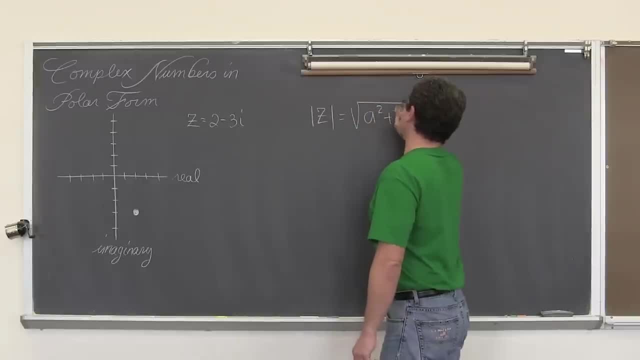 value is the square root of a squared plus b squared. Well, you might be going- that looks very, very familiar- to another formula I have learned, Which is: r is equal to the square root of x squared plus y squared. You would have seen this formula in a previous video. 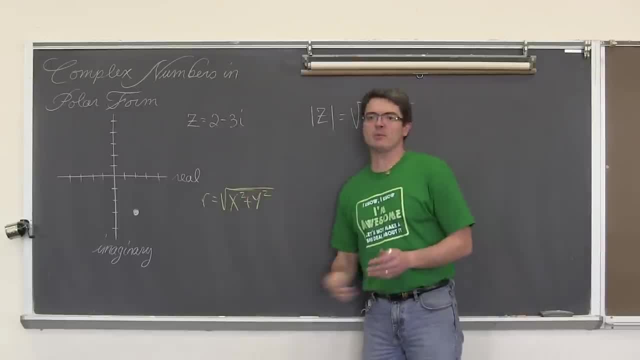 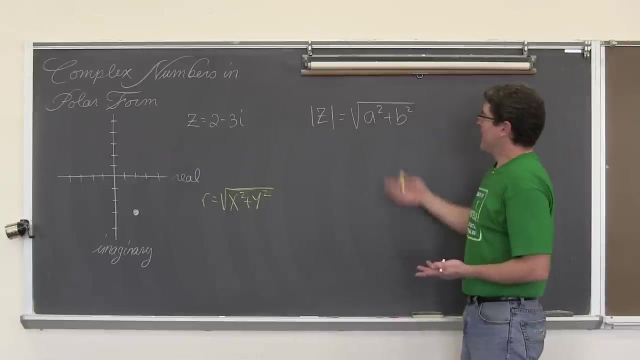 This formula. well, you have seen it probably since you started studying trigonometry, But we just did a video about converting between polar coordinates and rectangular coordinates And you know converting points and equations. This formula was in those videos, That is, and it is basically the Pythagorean Theorem, really, And these two formulas look exactly. 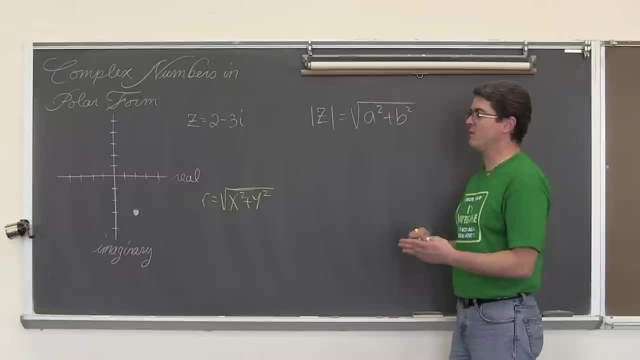 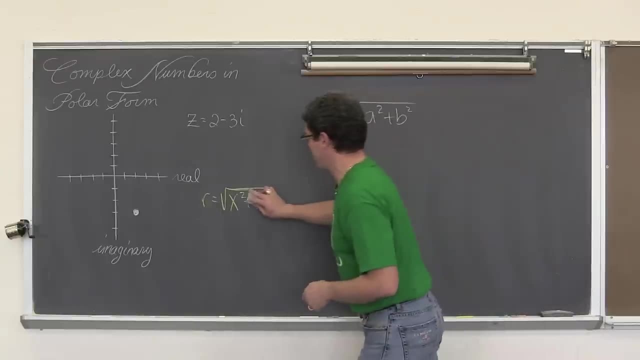 the same, except for, instead of dealing with real values, we are dealing with the imaginary and the real values. These are complex numbers, And so we are going to try to find the absolute value of z. Ok, Ok, So we are going to take x squared out and y squared out And replace them with the values. 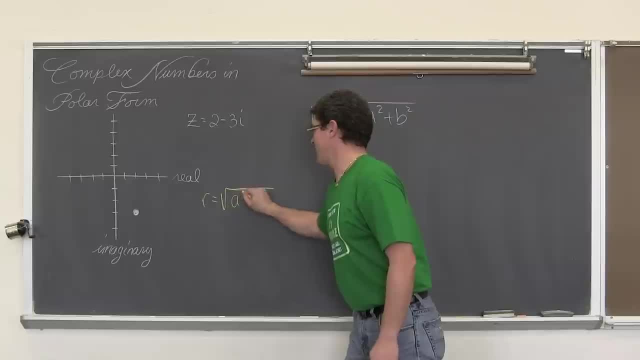 of x squared plus y squared, So it will be a squared plus b squared, And indeed I am going to make- well, let's just do it now. r equals the square root of a squared plus b squared. There is another formula that we learned and we have known for quite a while. 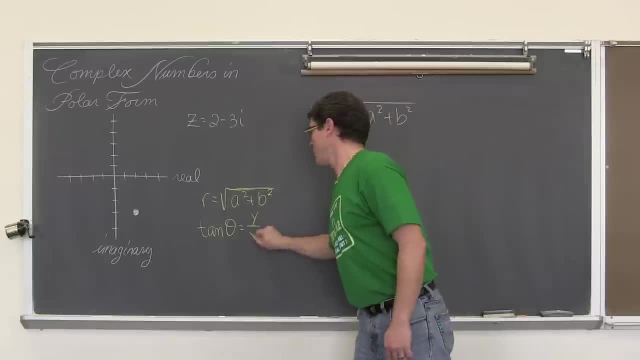 now in trig, which is the tangent of theta, is y over x. Well, those labels are good for a rectangular form of real values, but since we are using complex values, and it is real, imaginary, or what moves horizontally and what moves vertically, is going to be b over a. 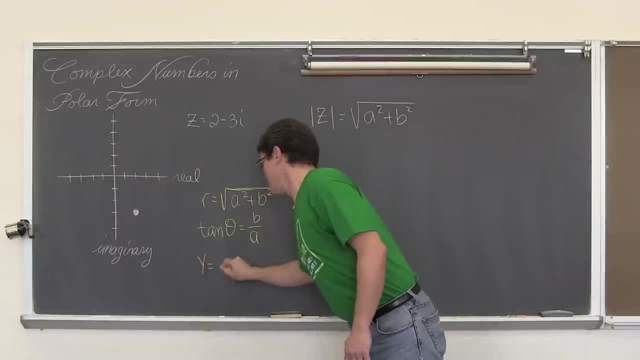 And let's see: y is equal to r sine theta. Well, y, the vertical movement in a complex number, is b, And then we have a, Ok Ok, So y is equal to r cosine theta. So we are kind of just really just changing the labels. 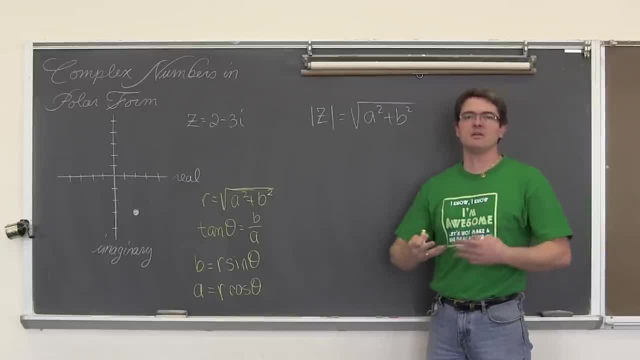 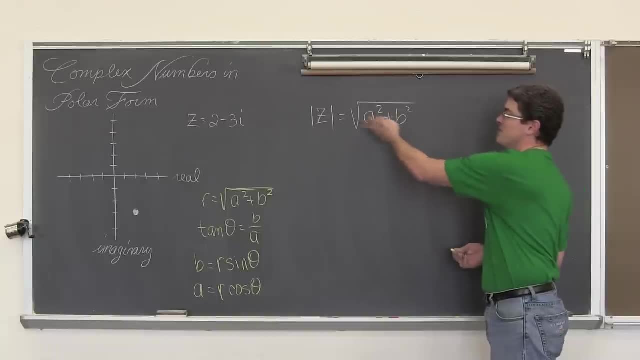 but yet everything is acting the same as it was in just the real rectangular coordinate plane, And the absolute value of a complex number is simply how far it is away from the origin. You should be recognizing this as either r or, again, the Pythagorean Theorem. 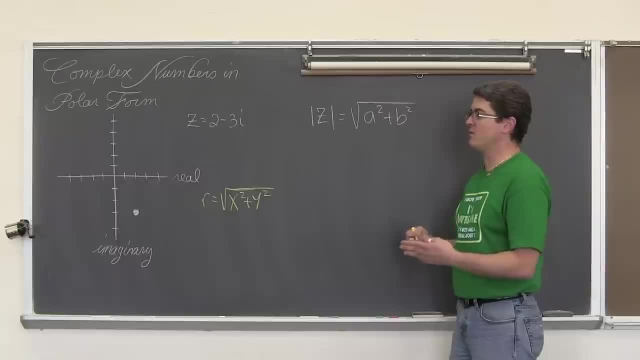 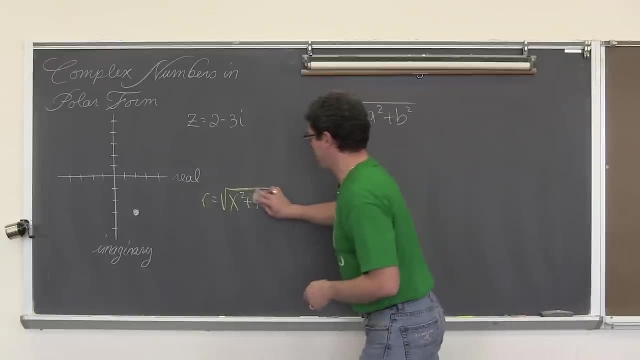 the same, except for, instead of dealing with real values, we are dealing with the imaginary and the real values, or these complex numbers, And so we are going to use these two formulas. Ok, Ok, So we are going to take x squared out and y squared out and replace them with the values. 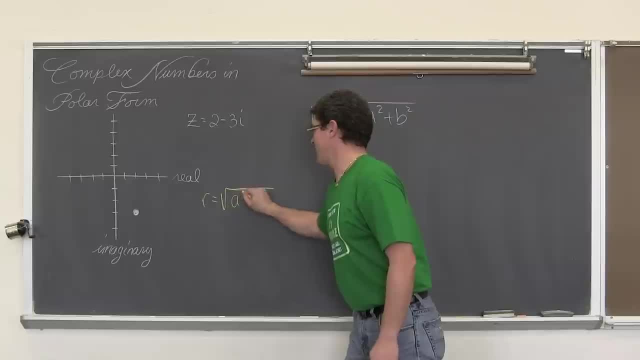 of x squared plus y squared, So it will be a squared plus b squared, And indeed I am going to make- well, let's just do it now. r equals the square root of a squared plus b squared. There is another formula that we learned and we have known for quite a while. 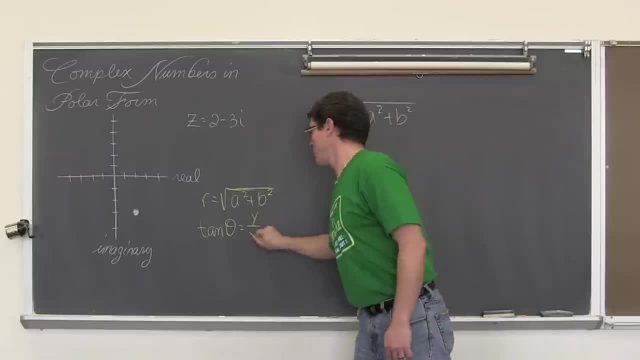 now, in trigonometry, which is, the tangent of theta is y over x. Well, those labels are good for rectangular equations, But what we are going to do is we are going to use the rectangular form of real values, But since we are using complex values, and it is real, 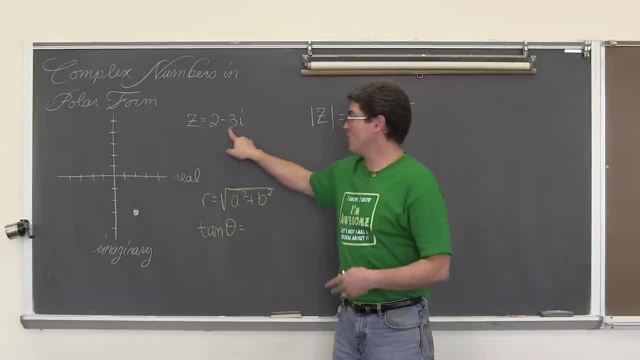 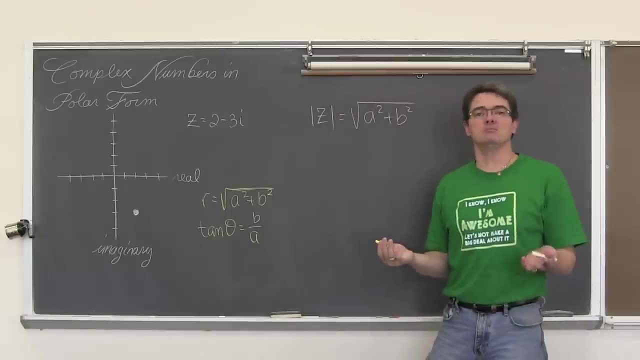 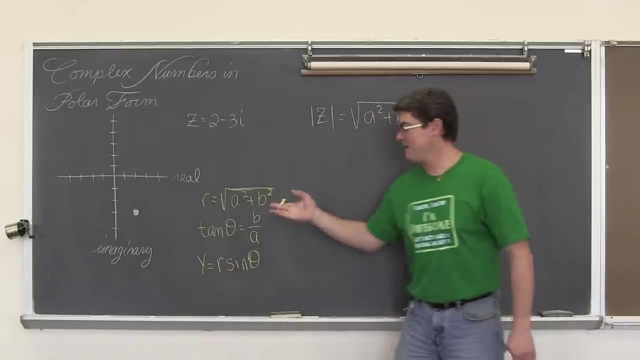 imaginary, or what moves horizontally and what moves vertically is going to be b over a. And let's see: y is equal to r sine theta. Well, y, the vertical movement in a complex number, is b, And then we have a over b. Ok. 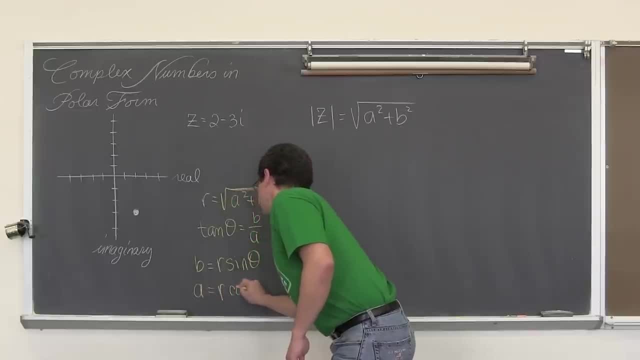 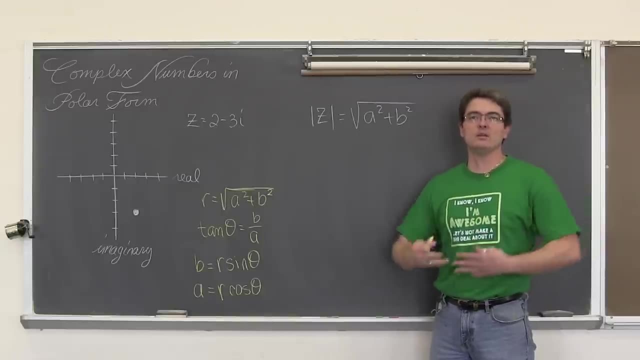 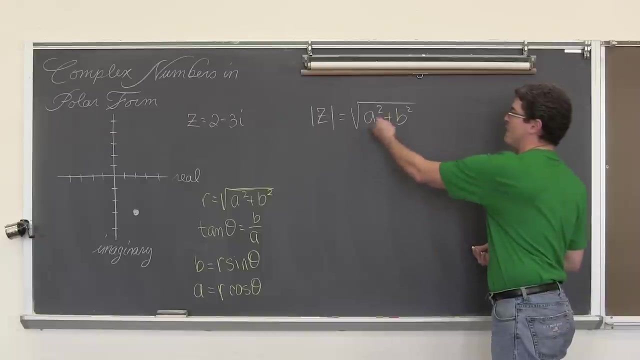 Ok, So we have a is equal to r, cosine, theta, So we are kind of just really just changing the labels, but yet everything is acting the same as it was in just the real rectangular coordinate plane, And the absolute value of a complex number is simply how far it is. 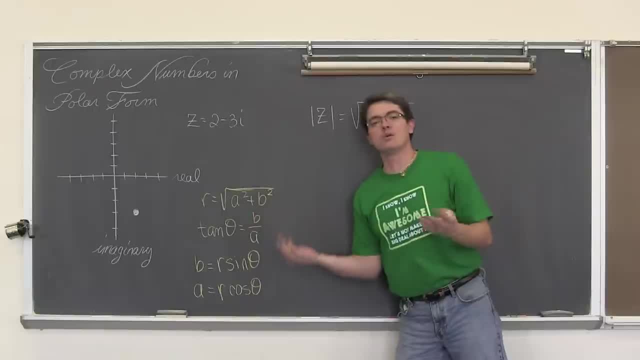 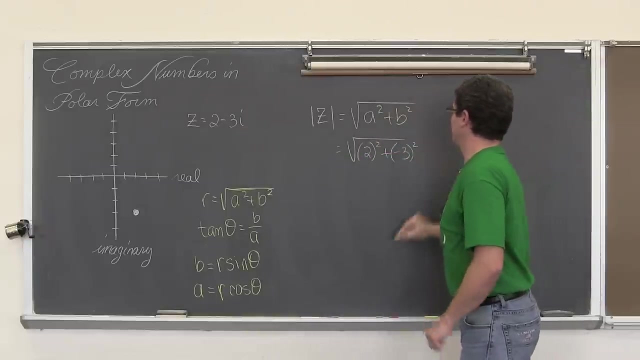 away from the origin. You should be recognizing this as either r or, again, Pythagorean Theorem. So this comes out to be the square root of a, the real part. two squared plus b squared, Ok, The imaginary coefficient of negative three. That comes out to be the square root of two. 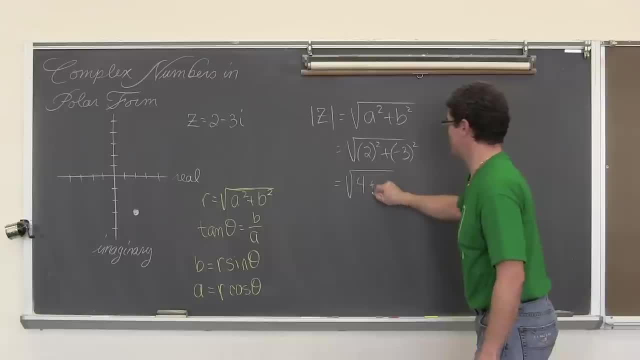 squared is four minus negative three squared, excuse me- plus negative three squared, which is nine, or the square root of thirteen. So the absolute value of z in this example is: Oh, I forgot my absolute value symbols. Ok, Absolute value is the distance that the point is away from the origin. And as a distance, 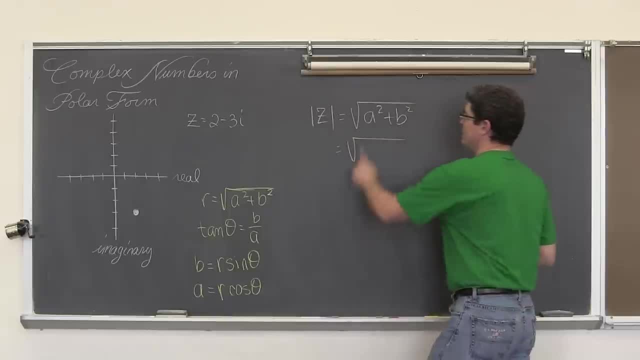 So this comes out to be the square root of a, the real part, two squared plus b. squared Plus b, the imaginary coefficient of negative three That comes out to be the square root of two squared, is four minus negative three squared, excuse me, plus negative three squared. 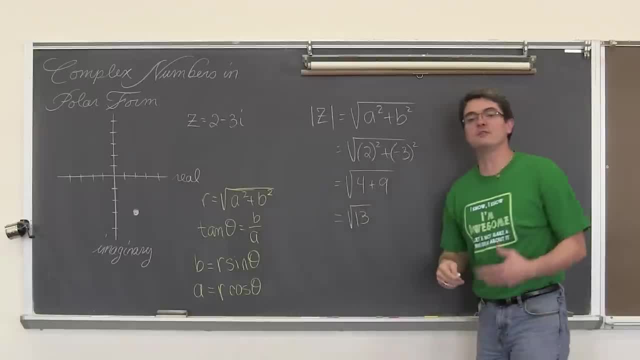 which is nine, or the square root of thirteen. So the absolute value of z in this example is: Oh, I forgot my absolute value symbols. Ok, Ok, Ok, Ok. So the absolute value is the distance that the point is away from the origin And as 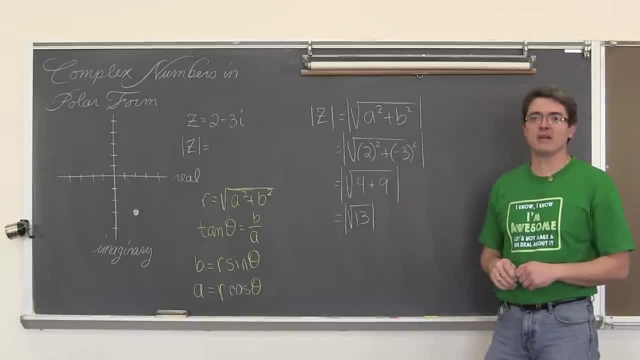 a distance. we want to make sure that comes out to be a positive answer, because the square root of thirteen could be positive or negative. three point something And we want to make sure we keep that positive answer. So the absolute value of z is going to be the square. 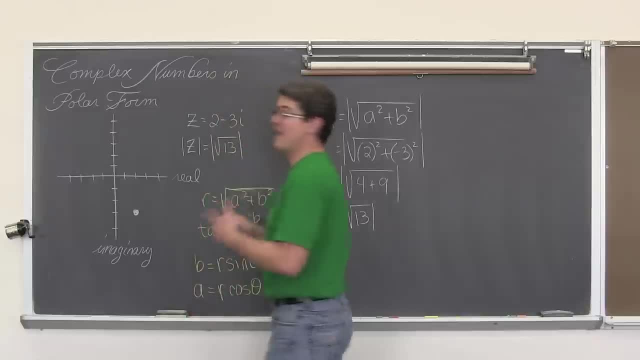 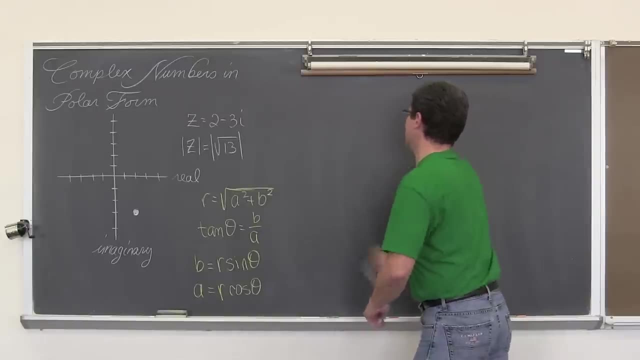 root of thirteen, Technically, the absolute value of the square root of thirteen. Ok, So that is how you find the absolute value of a complex number number. It is just really the distance that point is away from the origin. We have been. 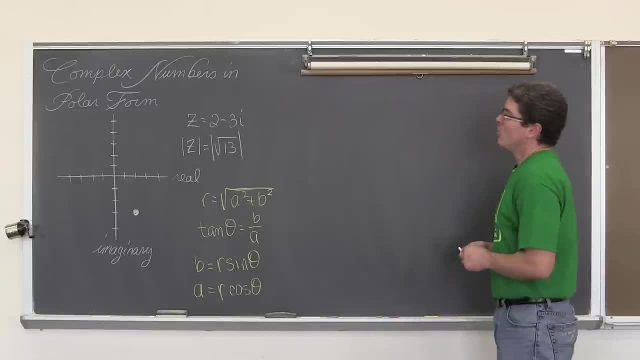 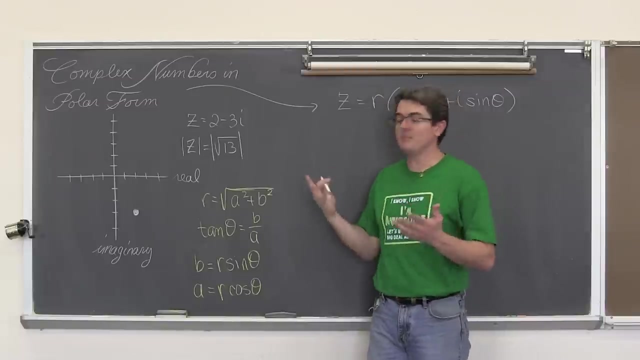 doing that kind of calculation now for a very, very long time. We are going to now introduce the formula to get this complex number into polar form. That is going to be: z is equal to r times the cosine of theta plus i sine theta. So how do we get 2 minus 3i, this imaginary 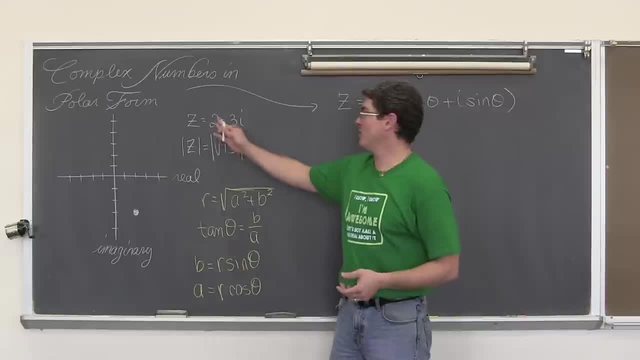 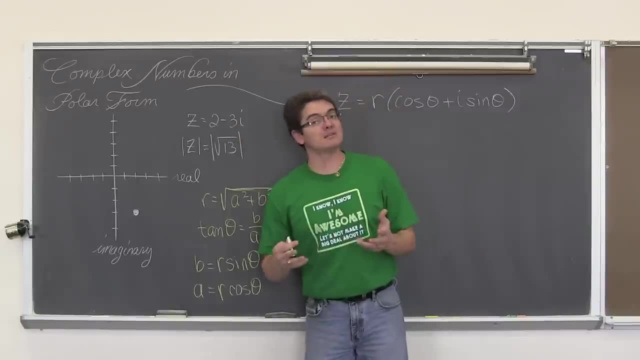 complex number into polar form. Well, we have a real portion acting very similar to an x value. We have an imaginary coefficient acting very similar to a y coordinate. We have these new conversion formulas which we recognize from converting between polar and rectangular form. Thus, getting this complex number into this polar form is going to be exact the same. 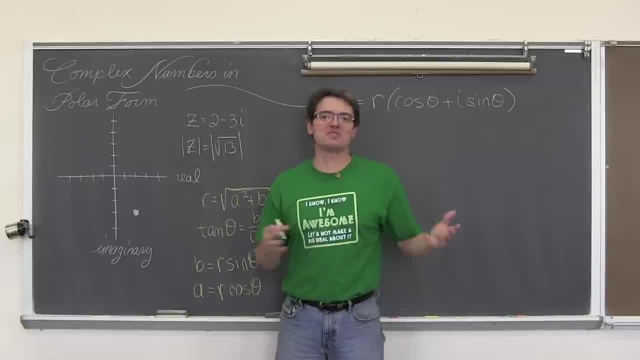 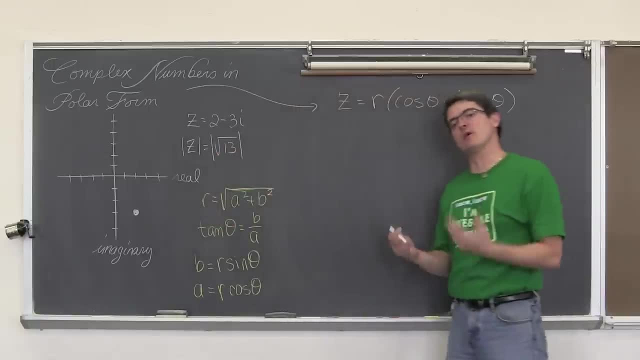 with this, different letters, as going from rectangular form to polar form, with just a regular coordinate. So, all that being said, we now know how far the point is away from the origin square to thirteen units. Now we need to know what theta is. 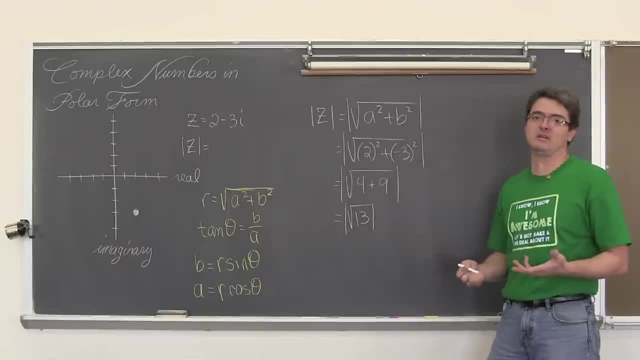 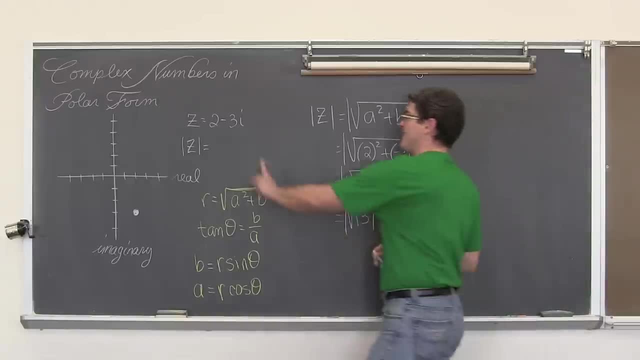 we want to make sure that comes out to be a positive answer Because you know, the square root of thirteen could be positive or negative. three point something And we want to make sure we keep that positive answer. So the absolute value of z is going to be the square. 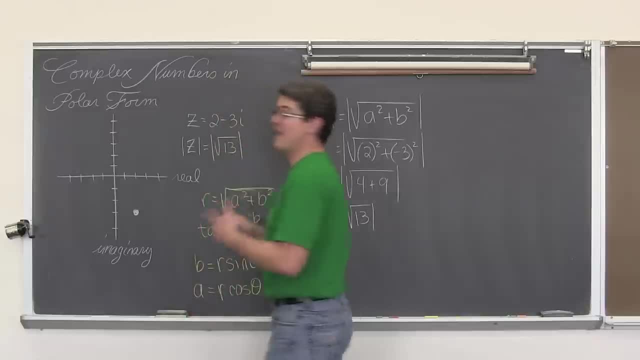 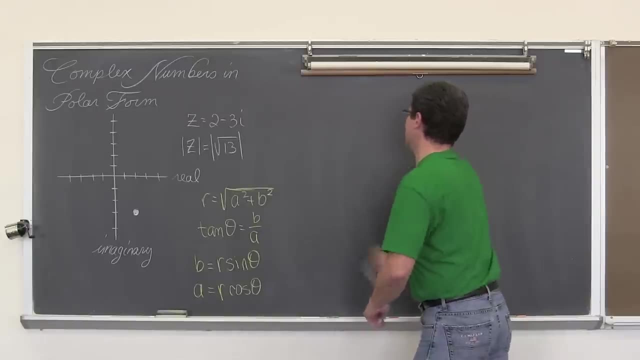 root of thirteen, Technically, the absolute value of the square root of thirteen. Ok, So that is how you find the absolute value of a complex number. it is just really the distance that point is away from the origin. We have been doing that kind of calculation now for a very, very long time. 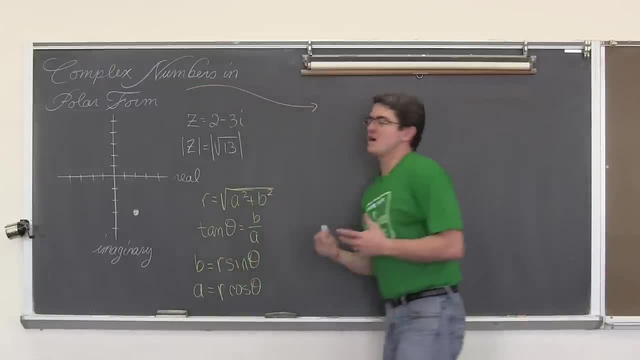 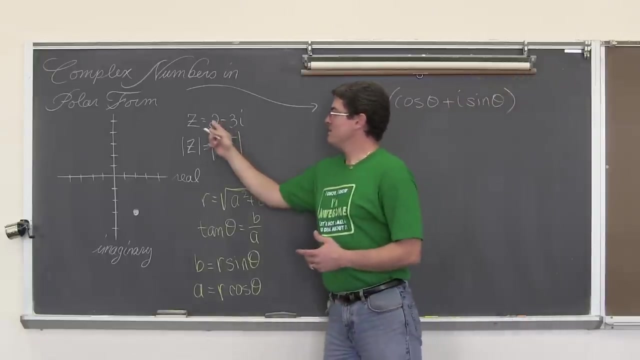 We are going to now introduce the formula to get this complex number into polar form, And that is going to be z, is equal to r times the cosine of theta plus i sine theta. So how do we get 2 minus 3i, this imaginary complex number, into polar form? 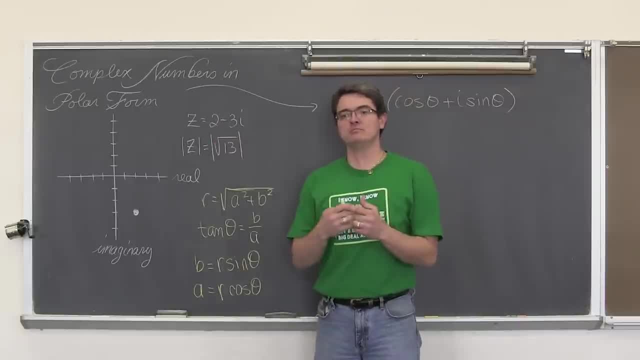 Well, we have a real portion acting very similar to an x value. We have an imaginary coefficient acting very similar to a y coordinate. We have these new conversion formulas, which we recognize from converting between polar and rectangular form And thus getting this complex number into this polar form. 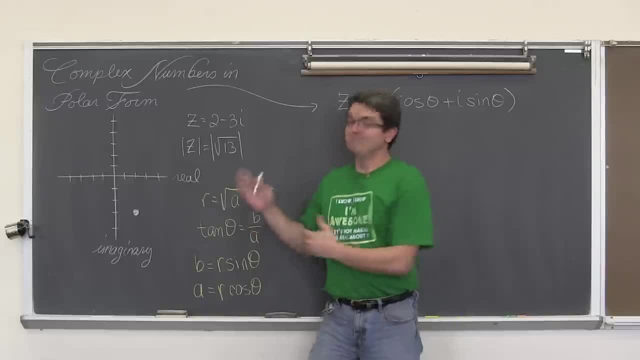 Is going to be exactly the same, with different letters, as going from rectangular form to polar form, with just a regular coordinate. So, all that being said, we now know how far the point is away from the origin square to 13 units. 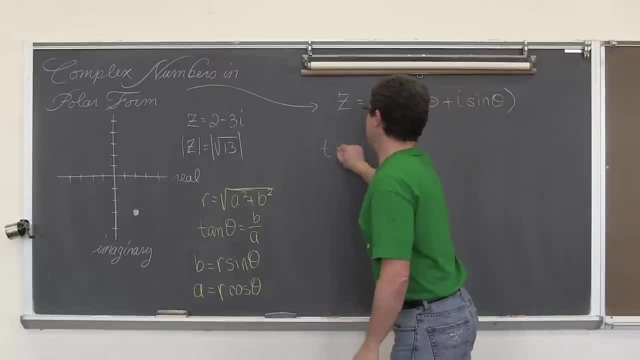 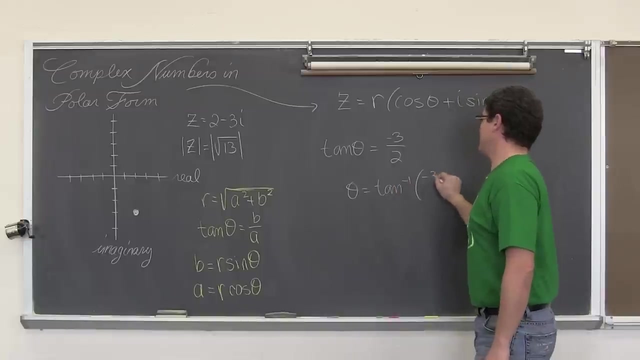 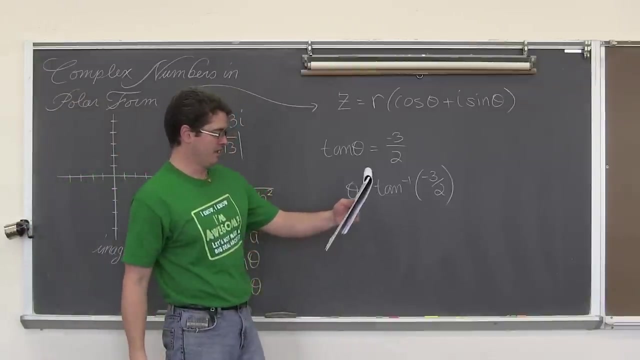 Now we need to know what theta is. So the tangent of theta is equal to y, which is or b negative 3 over 2.. And theta is equal to. therefore the inverse tangent of negative 3 halves, And off the top of my head, that comes out to be. where is it at? 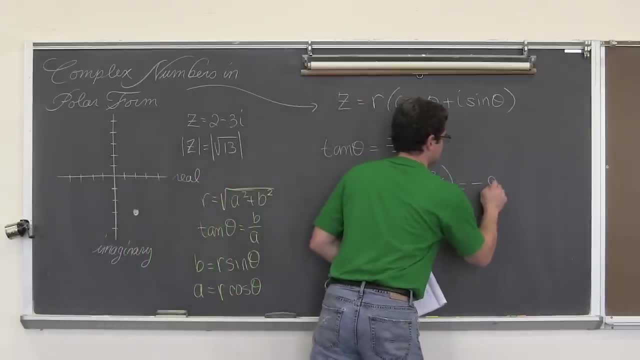 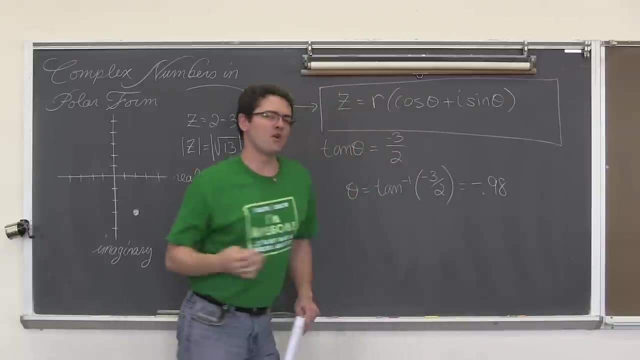 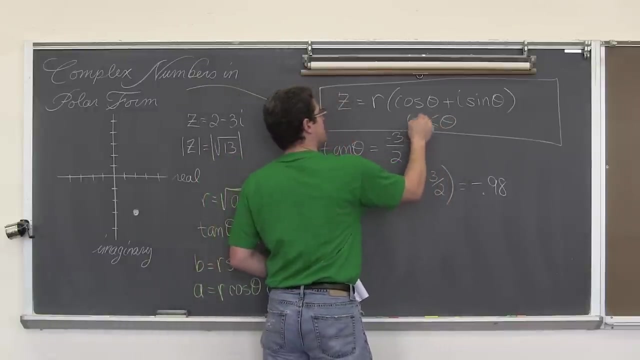 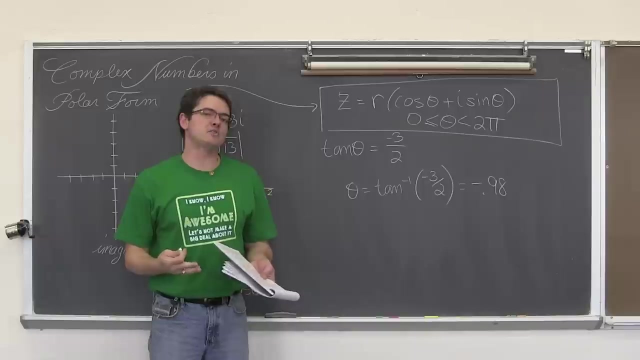 Negative: .98.. Now, one thing I just forgot. good thing, I picked up my notes here. This formula for writing a complex number in polar form is defined as theta being the angle between 0 and 2pi. But you can also have- well, not, but it can also be defined between 0 and 360, if you are. 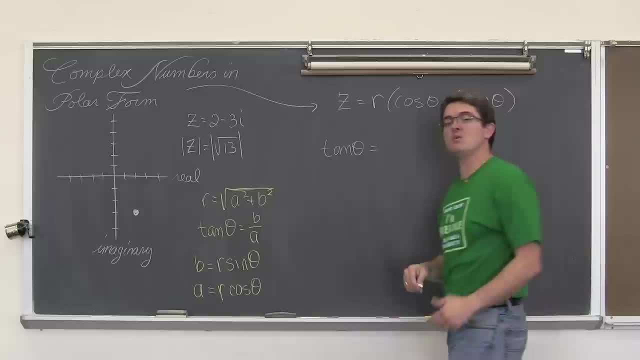 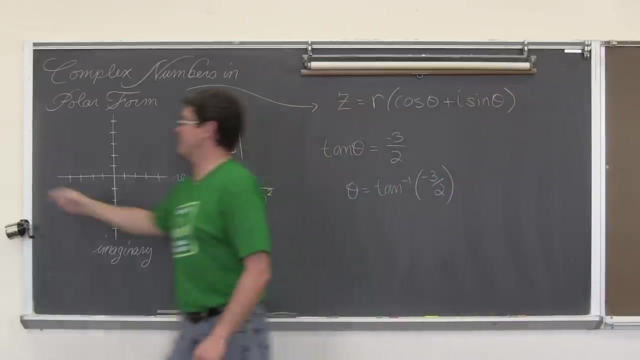 So the tangent of theta is equal to y, which is or b, negative three over two, and theta is equal to, therefore, the inverse tangent of negative three-halves, and off the top of my head that comes out to be where is it at? 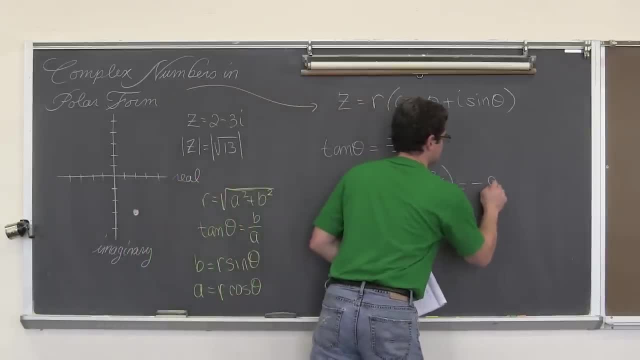 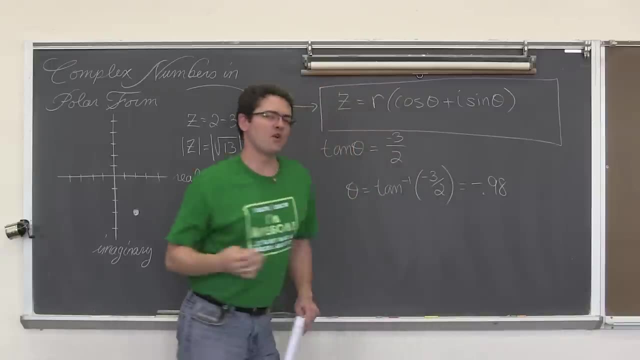 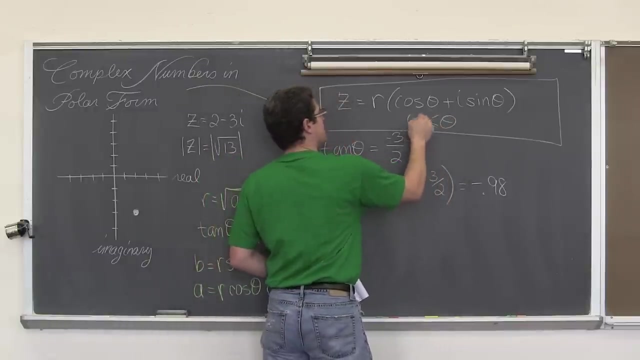 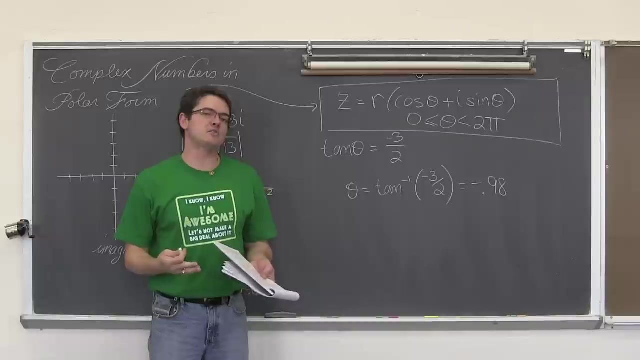 Negative point: nine-eight. Now one thing I just forgot. good thing, I picked up my notes here. This formula for writing a complex number in polar form is defined as theta being between zero and one, Zero and two-pod. but you can also have well, not, but it can also be defined between zero. 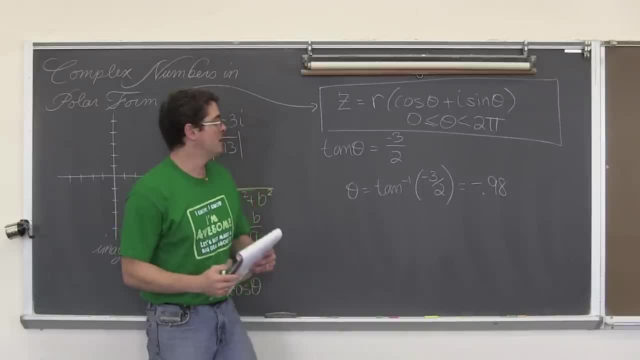 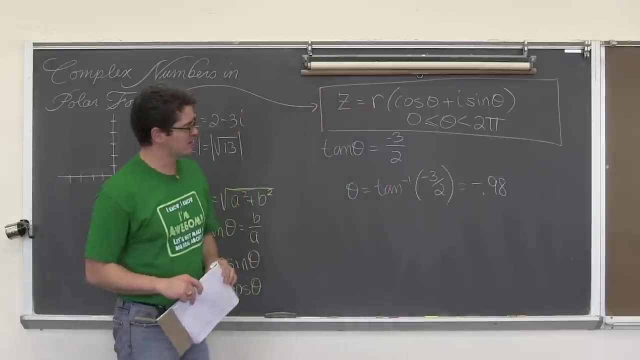 and three-sixty. if you are working in degrees, You can do these in degrees or radians. I have this defined as radians and that just means I am going to have to refer to my notes a little bit as I make sure I get the correct answer here. 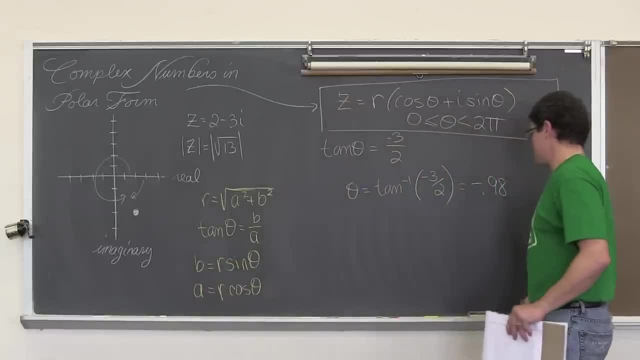 Ok, so what I want to do is, since this is in quadrant four, I want an angle that is in quadrant four, that has the same angle, The same reference angle of point nine-eight radians. So theta is going to be two pi or that one full rotation six point two-eight minus point. 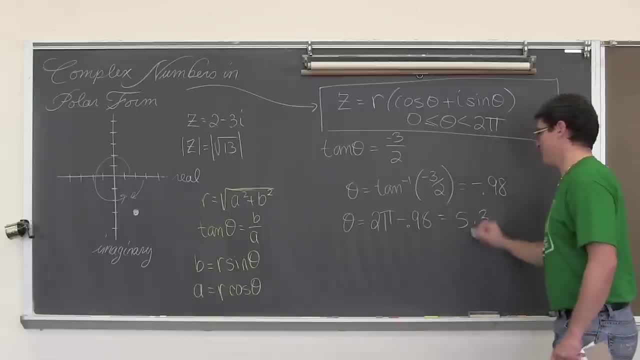 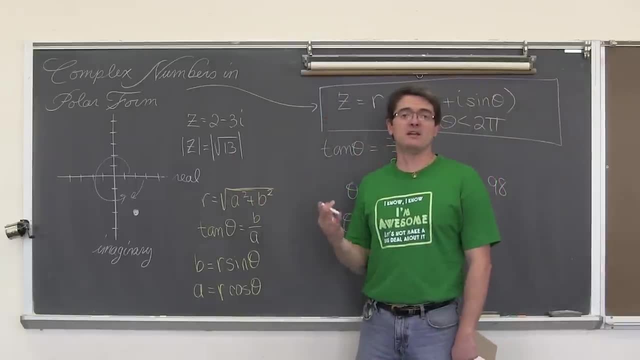 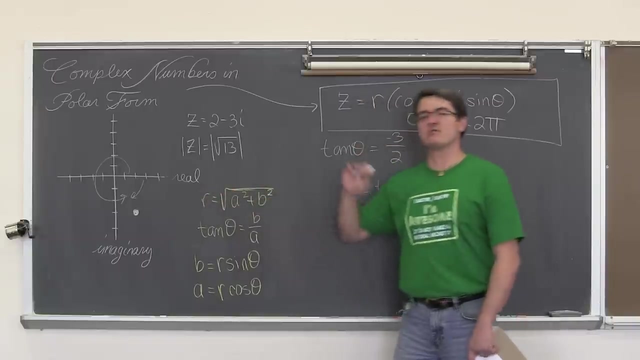 nine-eight, And that comes out to be five point three radians, I believe. yes, ok, So we found the absolute value of z, which was basically finding r. it was finding r as well. The absolute value of a complex number is the distance from the origin. r is the distance. 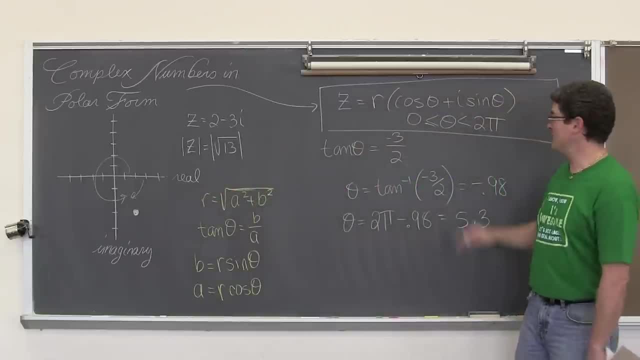 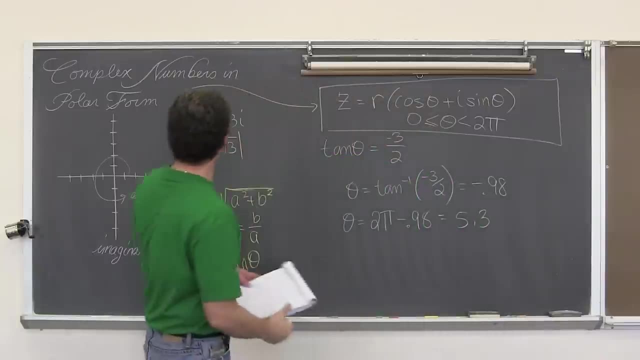 from the origin. So now we have r And we have theta, again defined between zero and two pi. We don't want that negative rotation, at least as this is defined. So this complex number in polar form is: drum roll please. square root of thirteen. 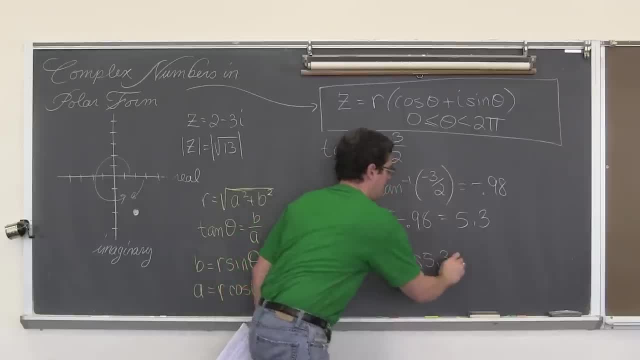 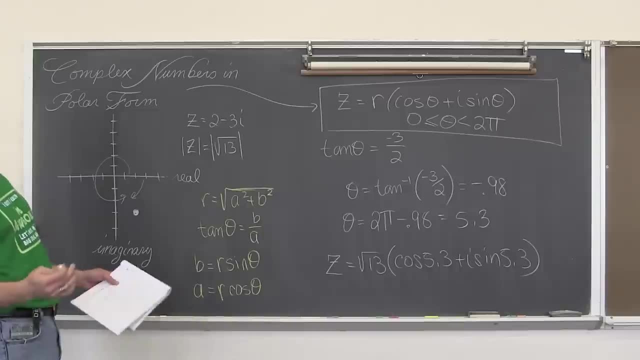 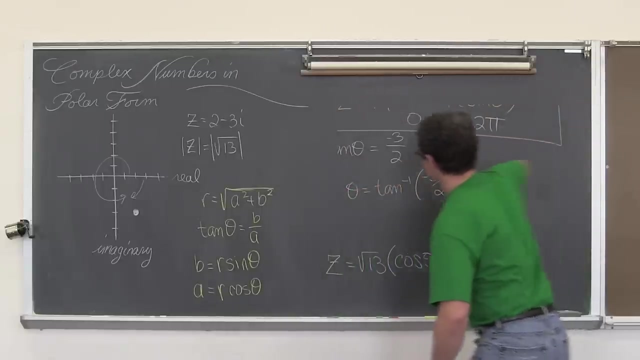 times the cosine of five point three plus sine of five point three, BAM, Ok, Whatever. So now that we have this number in polar form, how can we take this polar form complex number and convert it back into rectangular form? Now we know it is two minus three. i. 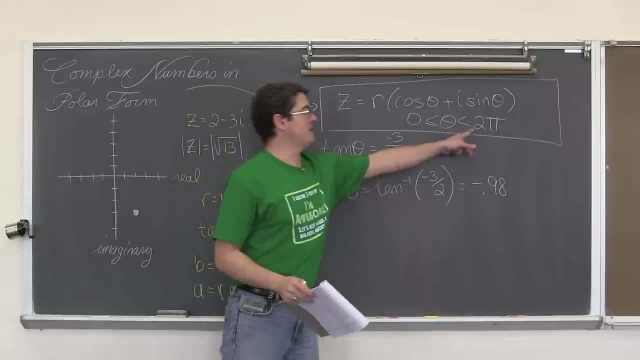 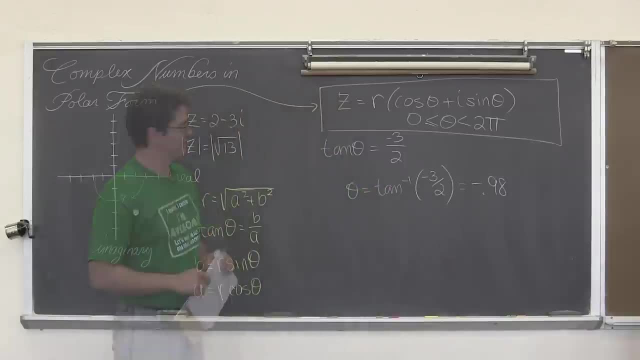 working in degrees. You can do these in degrees or radians. I have this defined as radians And that just means I am going to have to refer to my notes a little bit as I make sure I get the correct answer here. Ok, So what I want to do is: since this is in quadrant 4, I want an angle that is in quadrant. 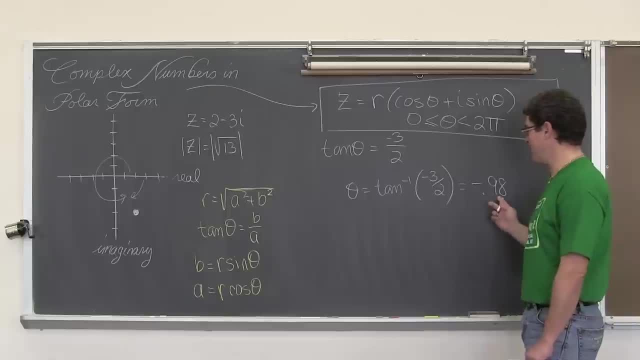 4. that has the same reference angle of .98 radians. So theta is going to be 2pi or that one full rotation, 6.28 minus .98.. And that comes out to be 5.3 radians, I believe. 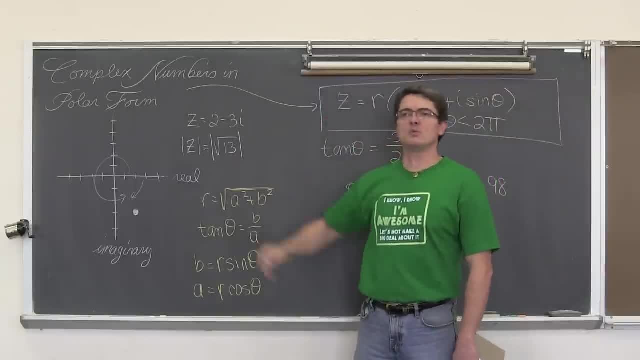 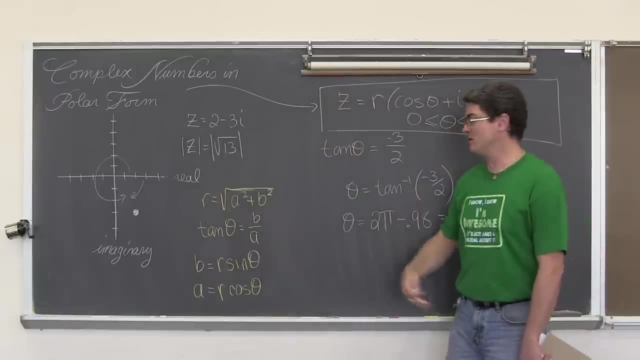 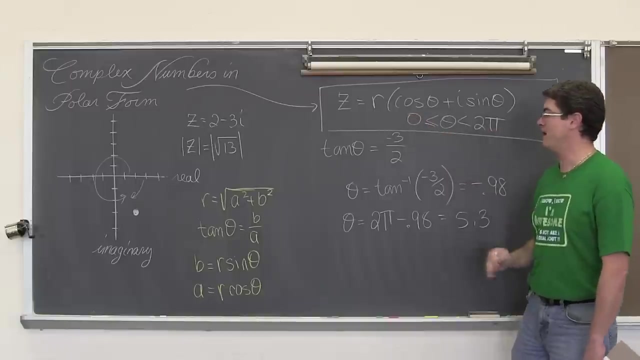 Yes, Ok, So we found the absolute value of z, which was basically finding r. it was finding r as well. The absolute value of a complex number is the distance from the origin. r is the distance from the origin. So now we have r and we have theta, again defined between 0 and 2pi. 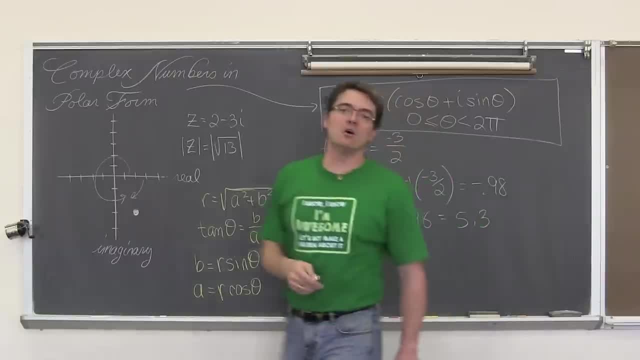 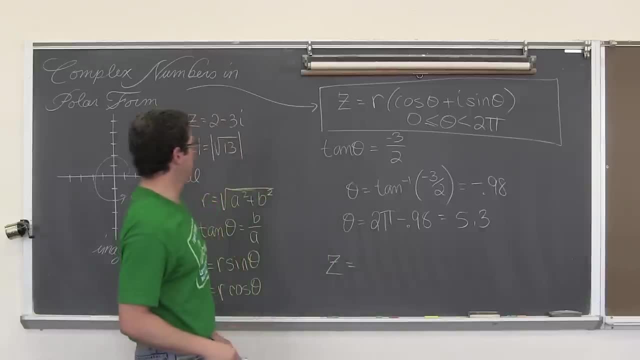 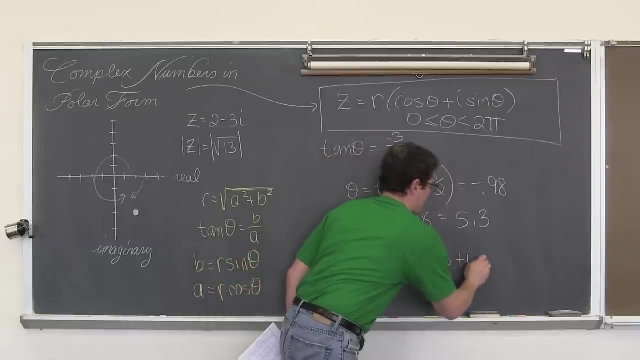 We don't want that negative rotation, at least as this is defined. So this complex number in polar form is: drum roll please. square root of 13 times the cosine of 5.3 plus times the sine of 5.3.. BAM. 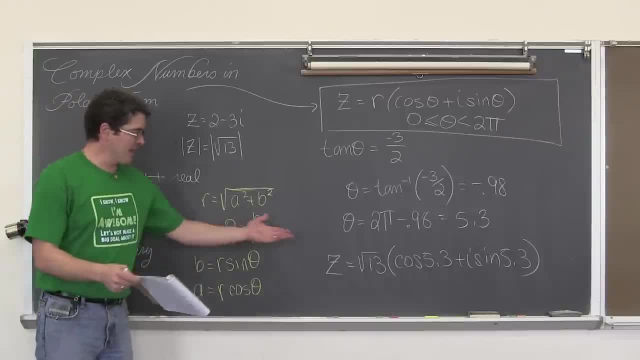 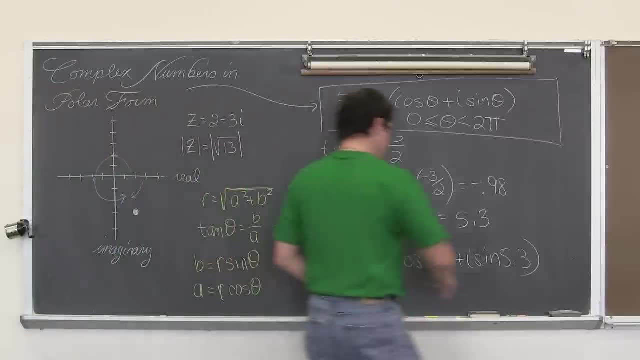 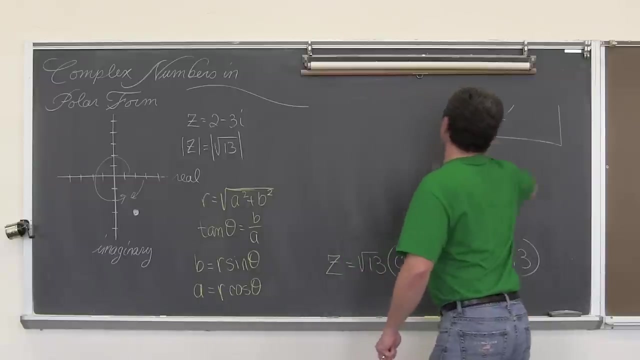 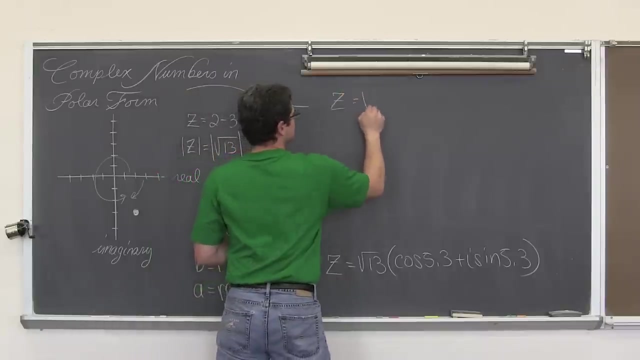 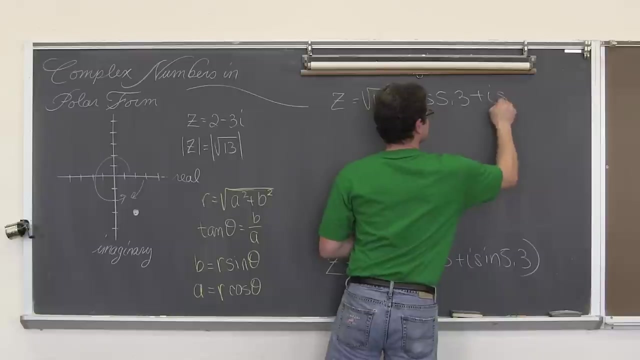 Ok, Whatever. So now that we have this number in polar form, how can we take this polar form complex number and convert it back into rectangular form? Now we know it is 2 minus 3i, Ok, Ok. Ok, Now we go into a regular rectangular form. 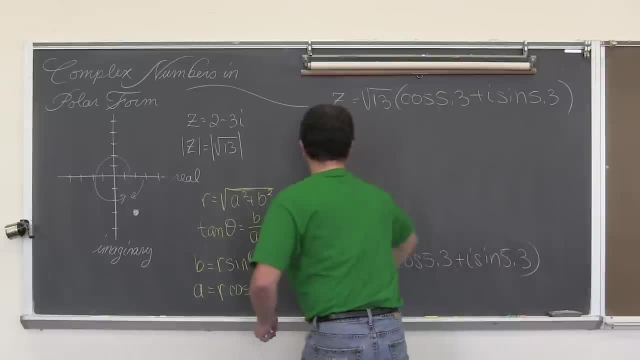 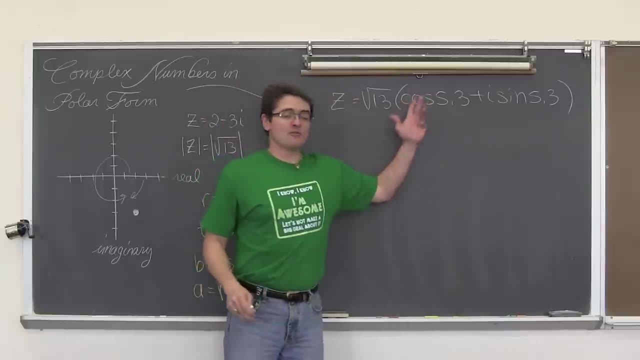 So we are going to do this drill, but how do we take this number in polar form, this complex number that is in polar form, and convert it back into just regular rectangular form? How do we even know that it is in polar form to begin with? 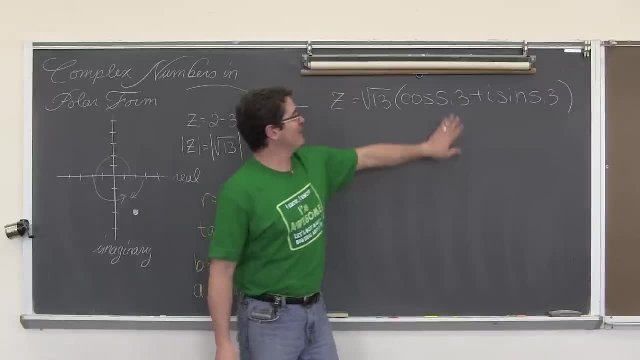 Well, it has trig functions in it. And how do I know these are not degrees, Because I don't see little degree marks. There is no symbol for radians, It just lights up. Ok, whatever, It is just there. Well, if you remember how to convert between polar coordinates and 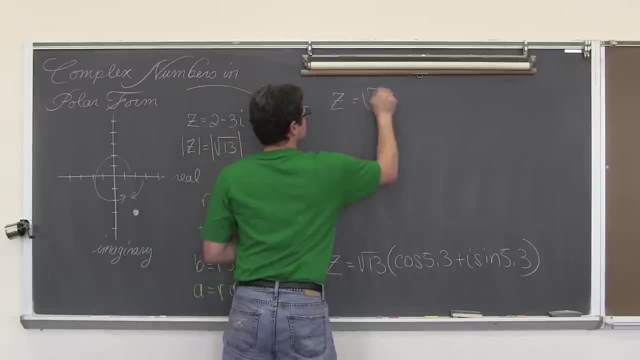 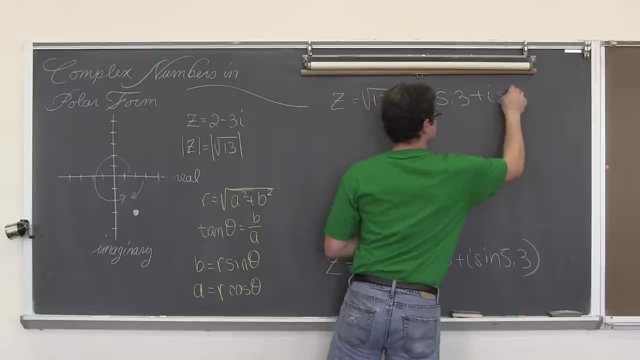 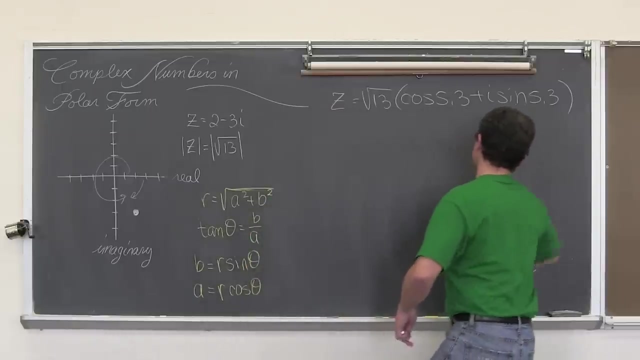 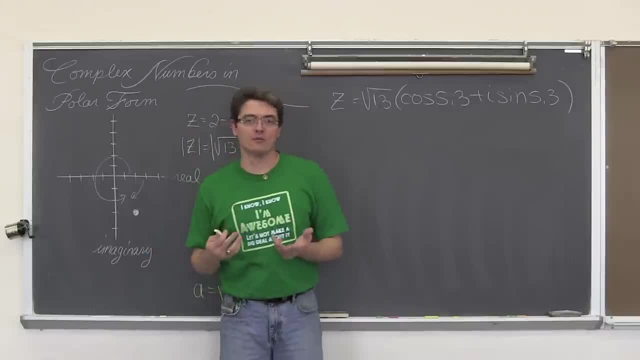 polar form and convert it back into just regular rectangular form. How do we even know that it is in polar form to begin with? Well, it has trig functions in it. And how do I know these are not degrees? Because I don't see little degree marks. 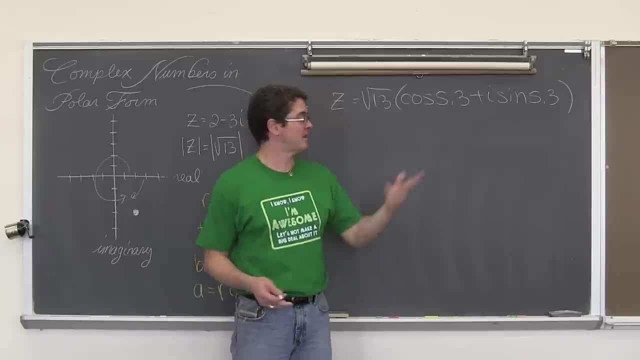 There is no symbol for radians, Just whatever was just there. Well, if you remember how to convert between polar coordinates and rectangular coordinates, you remember that going from rectangular to polar was very simple. Whatever the calculator spit out was the answer, Because your calculator can only deal with functions. 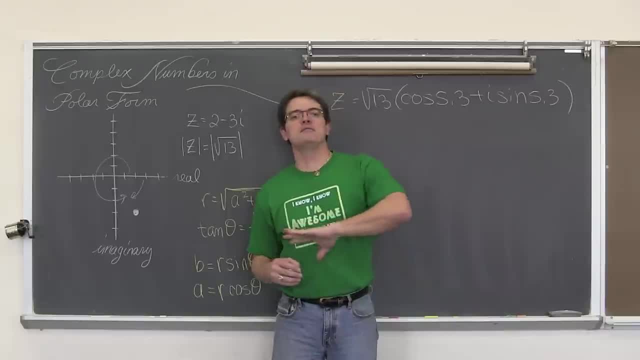 again. I am repeating this So you can do the sine of any answer you want: The sine of 30 degrees, the sine of 80 degrees, the sine of 5pi over 3 radians, the sine of 8623 radians? Who cares? The sine function is a function. It moves along the x axis and 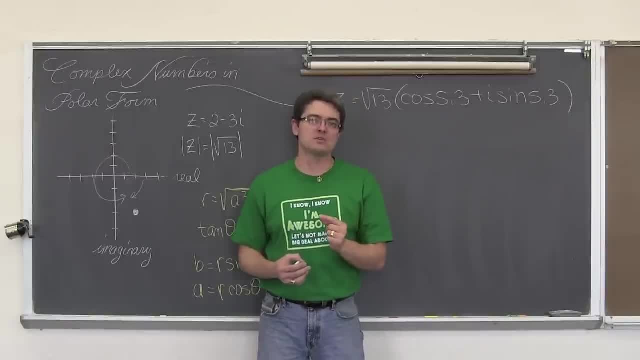 for every x there is only one y. But when you do inverse trig functions, as we did remember, we did the tangent of theta and we didn't get 5.3, we got negative, whatever it was, .98.. We have to play with those numbers a little bit, Because inverse trig functions 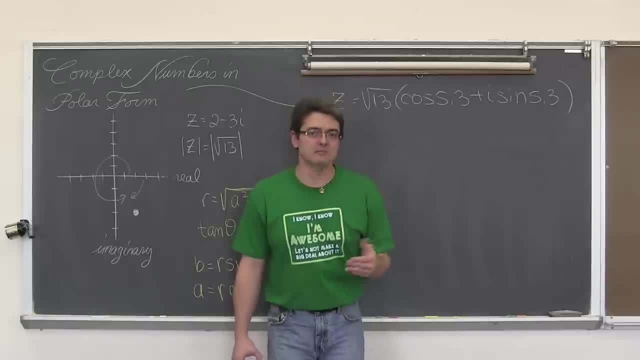 are not really inverse trig functions. They have to be restricted. So inverse tangent: negative 90, positive 90. Inverse cosine 0 to pi or 0 to 180.. Inverse sine only gives you negative 90 to positive 90 or negative pi over 2, positive pi over 2.. But you don't. 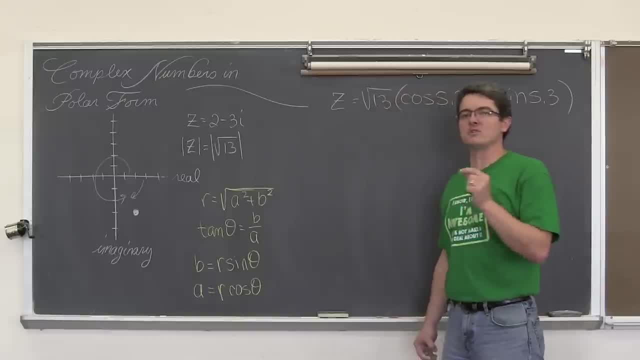 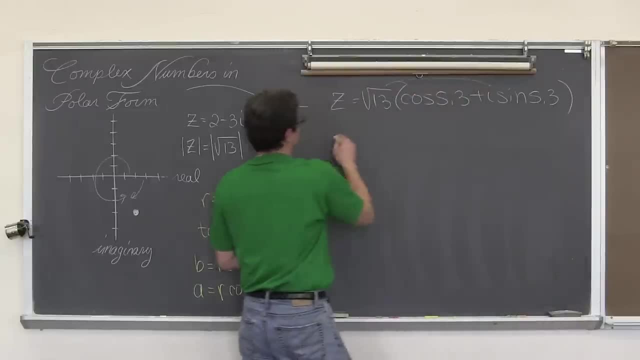 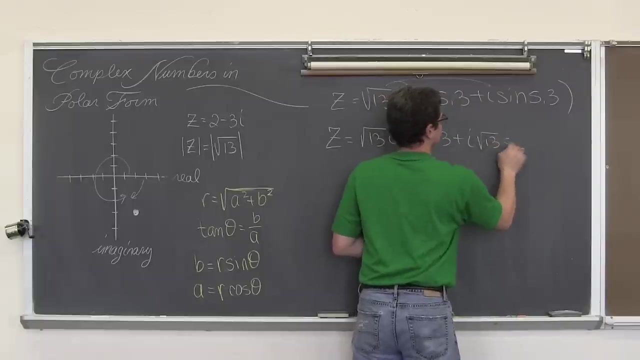 have that problem with regular trig functions. All your regular trig functions act as functions. So if you want to put this back into rectangular form, I would suggest just putting the square root of 13 back through or distributing the r value. Make sure your calculator is in the correct mode. If you are in radians, make sure you. 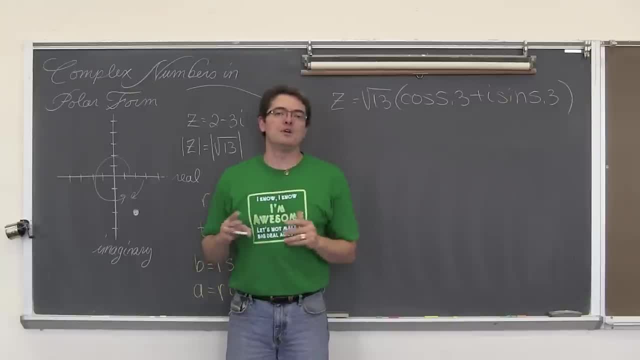 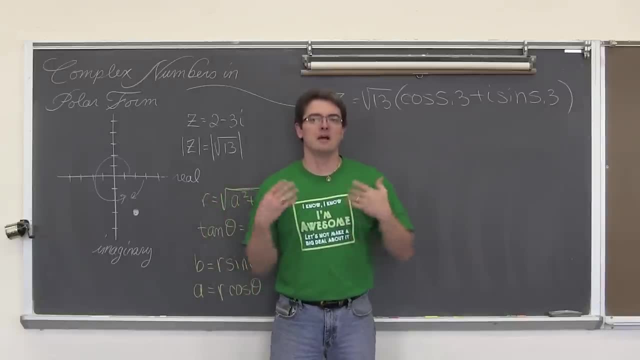 rectangular coordinates. you remember that going from rectangular to polar was very simple. Whatever the calculator spit out was the answer, Because your calculator can only deal with functions. Again, I am repeating this So you can do the sine of any answer you want. 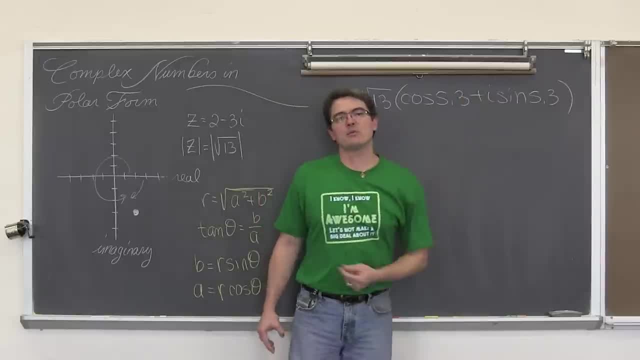 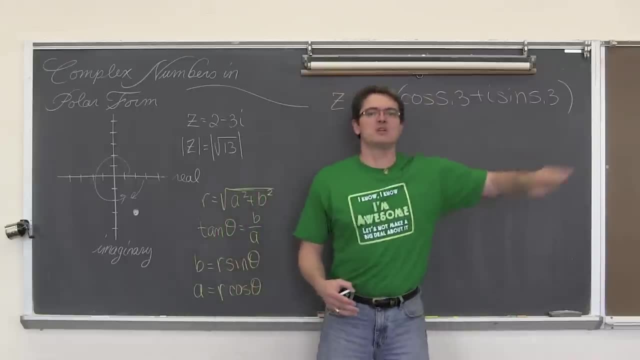 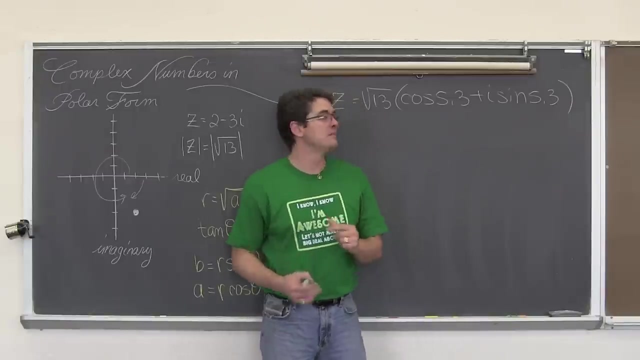 The sine of 30 degrees, the sine of 80 degrees, the sine of 5pi over 3 radians, the sine of 8623 radians? Who cares? The sine function is a function. It moves along the x axis and for every x there is only one y. But when you do inverse trig functions, as we did remember, 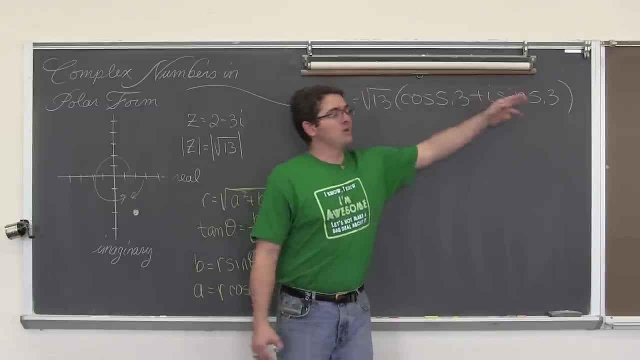 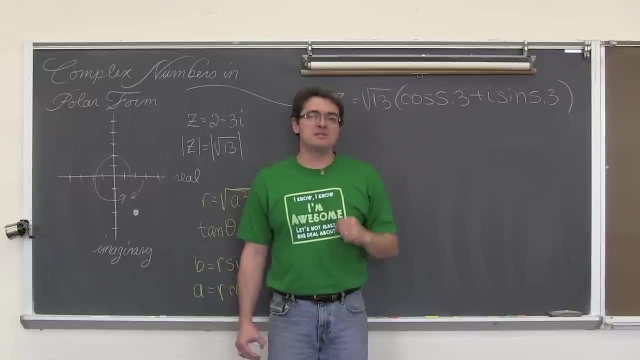 we did the tangent of theta and we did not get 5.3, we got negative, whatever it was .98.. We have to play with those numbers a little bit, Because inverse trig functions are not really inverse trig functions. They have to be restrictive. 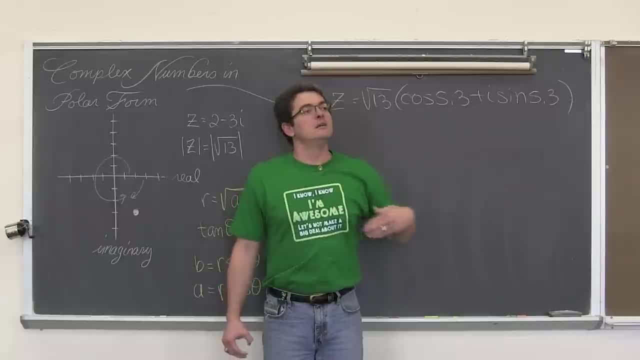 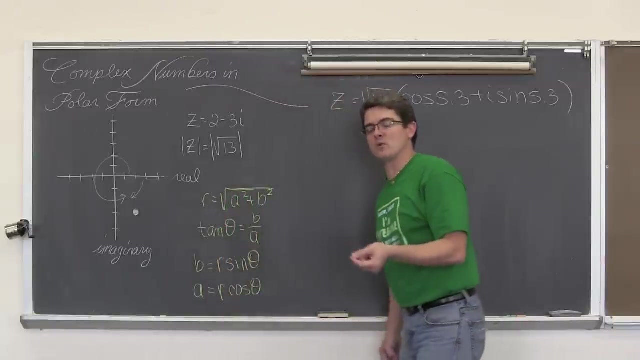 So inverse tangent negative 90, positive 90. Inverse cosine 0 to pi or 0 to 180.. Inverse sine only gives you negative 90 to positive 90. Or negative pi over 2, positive pi over 2.. But you don't have that problem with regular trig functions, All your regular. 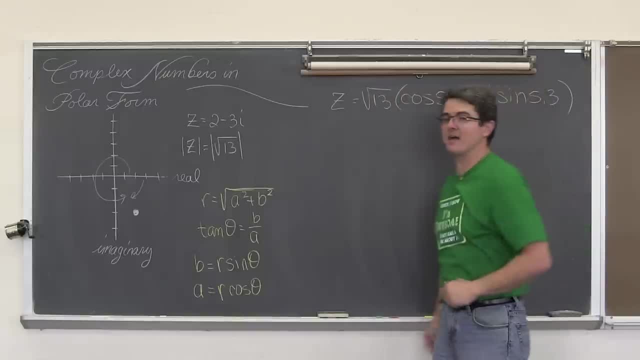 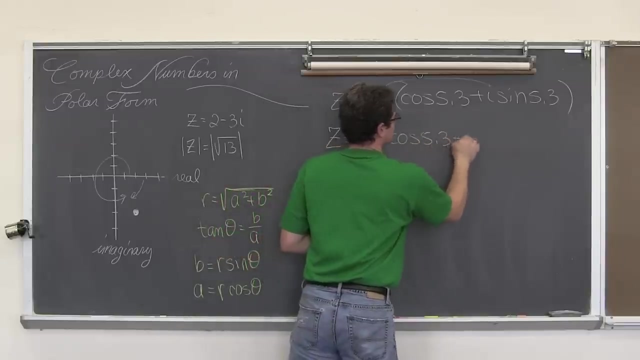 trig functions act as functions. So if you want to put this back into rectangular form, I would suggest just putting the square root of 13 back through or distributing the all r value. Make sure your calculator is in the correct mode If you are in radians. 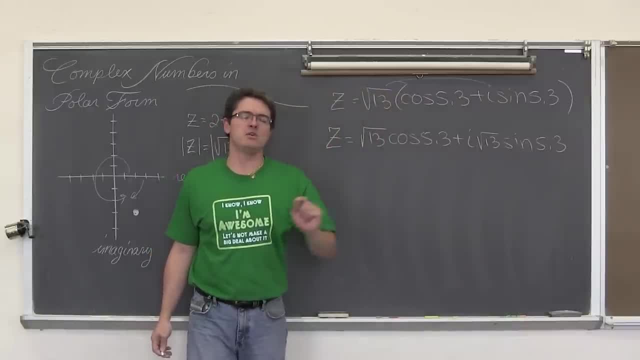 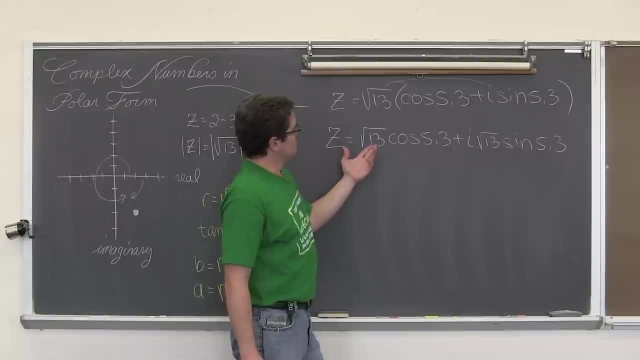 make sure you are in radian mode. Every time you hit sine cosine or tangent, you have to make sure your calculator is in the right mode, Otherwise it doesn't make any difference. So Take your calculator 13 times, the cosine of 5.3 is, as we know, 2. It might come out. 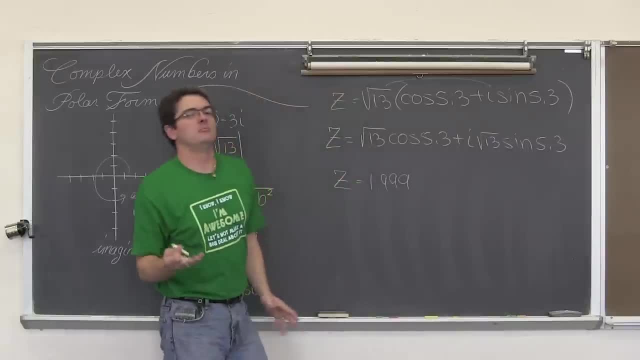 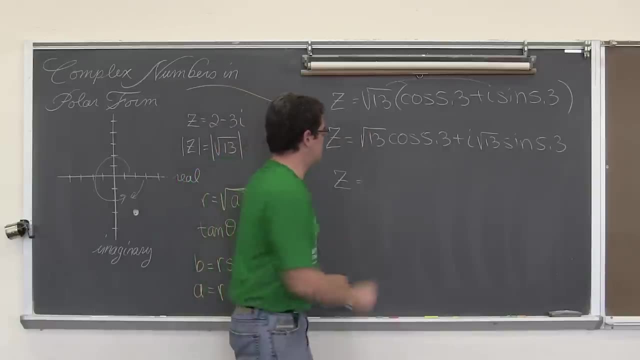 to be like 1.999,, but it is just round off error because I have only, you know, whatever, It is just round off error. So it is going to be basically 2, and then square root of 13 times the sine of 5.3 is negative 3i. So there you go Complex rectangular form into 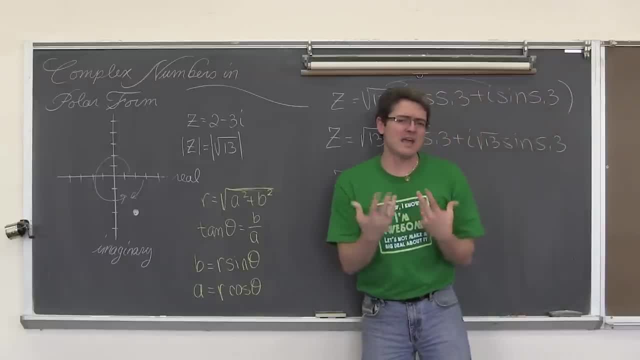 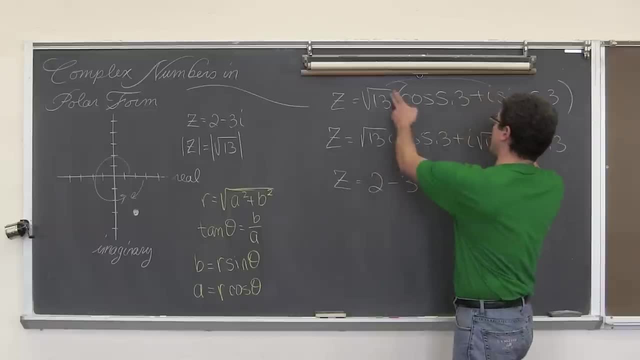 polar form steps. Make sure that the theta answer that you get from your calculator is probably not going to be the final answer, but it is a useable number When you go from polar form back into rectangular form. just type it in your calculator. Whatever comes out as the 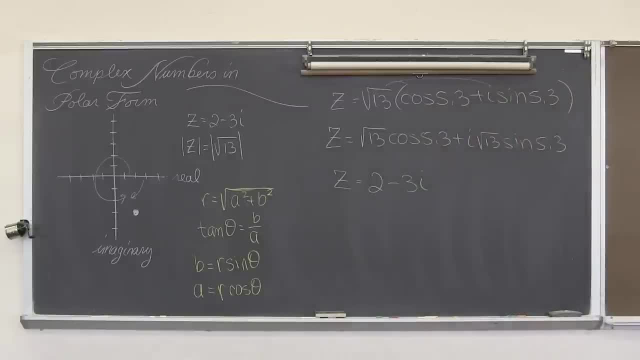 answer: BAM, I am Mr Tarrou. Go, Do Your Homework. 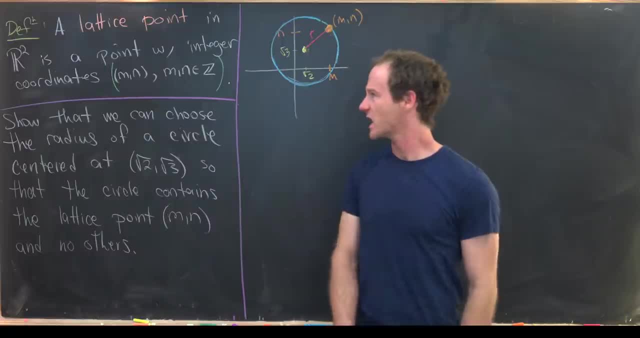 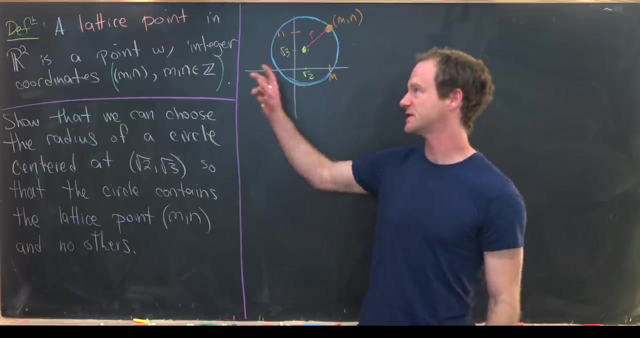 Here I've got a nice little geometry problem which, when you see the solution, it's not super surprising. But without looking deep into the calculation, I think it is a surprising result. So before we jump into what the problem is, let's recall a little bit of a definition. 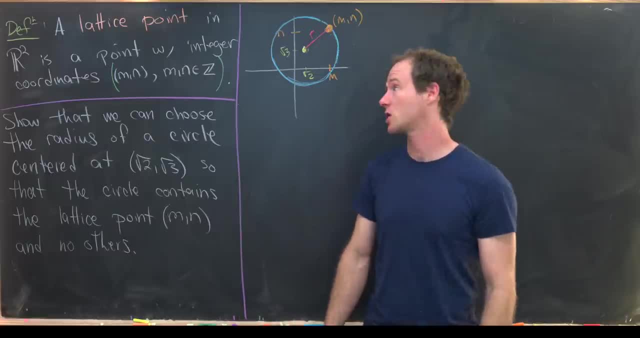 So if you consider the Cartesian coordinate, plane R2, a lattice point inside of the plane is a point with integer coordinates. So in other words, the x and y coordinate are both integers. So it's got the form mn, where m and n are integers. Then what's our goal? So our goal: 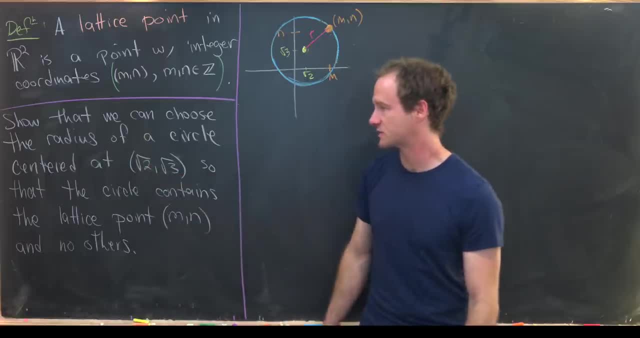 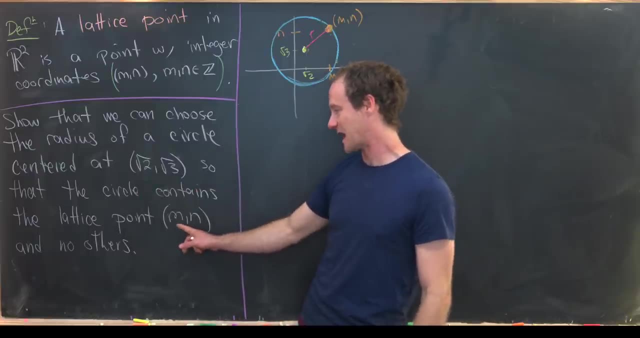 is to show that we can choose the radius of a circle centered at square root of 2, square root of 3, so that this circle contains the lattice point mn and no other lattice points. Notice that this lattice point is a point with a radius of a circle centered at square root of 2 square. 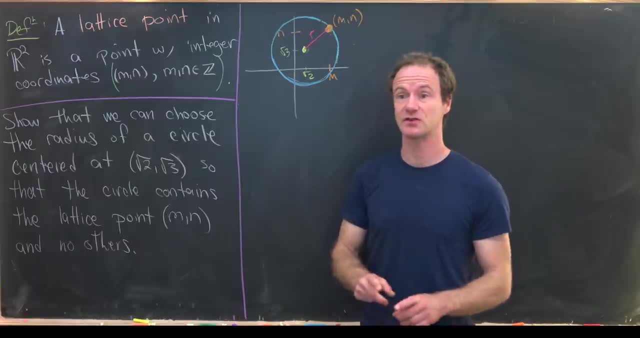 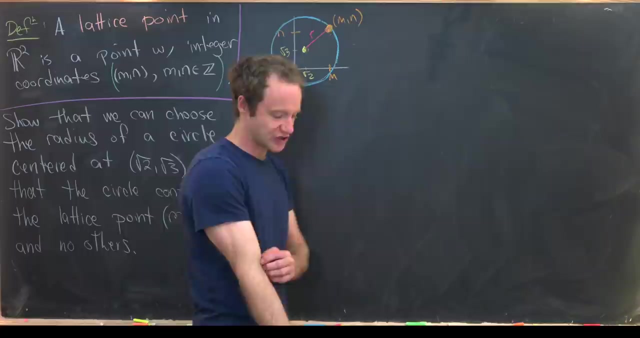 root of 3. This lattice point is general. That really means that we can have this circle achieve any lattice point that we want in the plane, but that circle only achieves that one lattice point and no other lattice point. Okay, so let's maybe look at a picture of the situation and then we'll 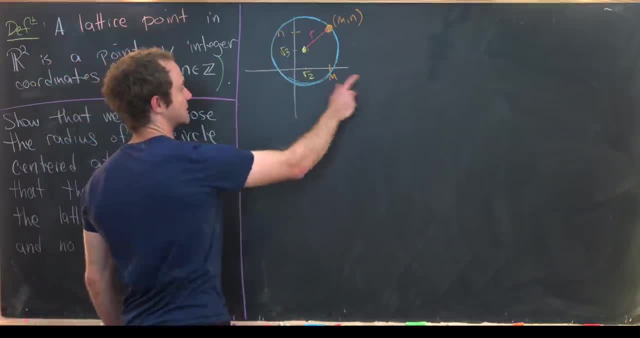 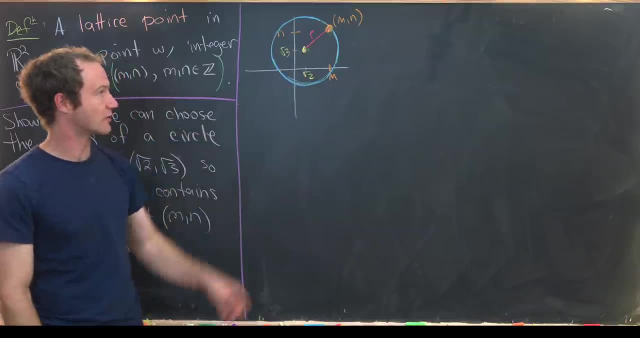 jump into the solution. So here I've got my Cartesian coordinate plane. here, So I've got my x-axis and my y-axis. I just sketched out this point: square root of 2, square root of 3.. And then I put this point, m comma n, as my lattice point. So this is m units from the origin in the.